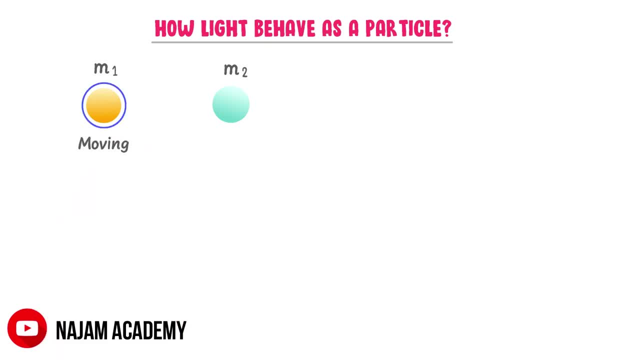 m1 and m2.. Let ball m1 is moving and ball m2 is moving. Let ball m1 is moving and ball m2 is moving to is stationary. We know that anything moving possesses two things: kinetic energy and momentum. So this ball possesses kinetic energy and momentum. Now this moving ball will head this. 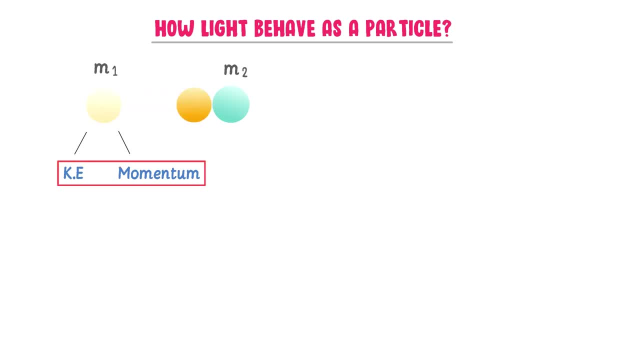 stationary ball and will transfer its kinetic energy and momentum to it. As a result, this ball will stop and this ball will start moving. From this example we learn that during collision- collision- particles transfer kinetic energy and momentum. Similarly, consider a metal. 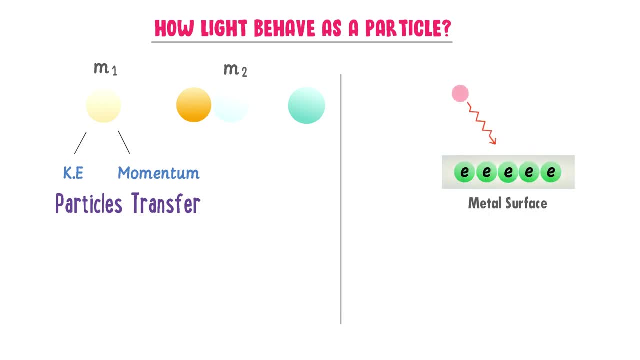 surface. We know that light travels in discrete wave packets, quanta, or photons, which we have already learned in Planck's quantum theory, and its link is given in the description. When this photon of light hits this electron of the metal, it will transfer its kinetic 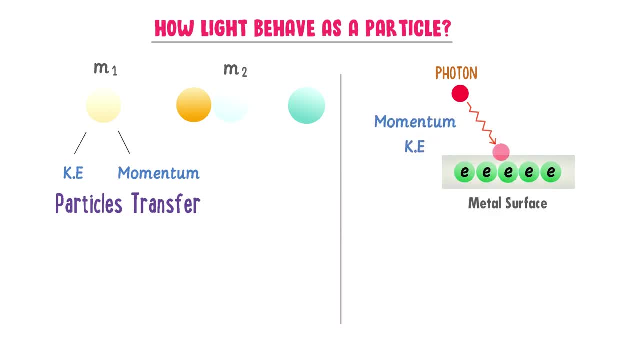 energy and momentum to this electron Subtitles by the Amaraorg community. As a result of this collision, the electron would be ejected from the metal surface. Here, differing collision between two particles causes the transfer of kinetic energy and momentum. Similarly, here, differing collision between photon and electron causes the transfer. 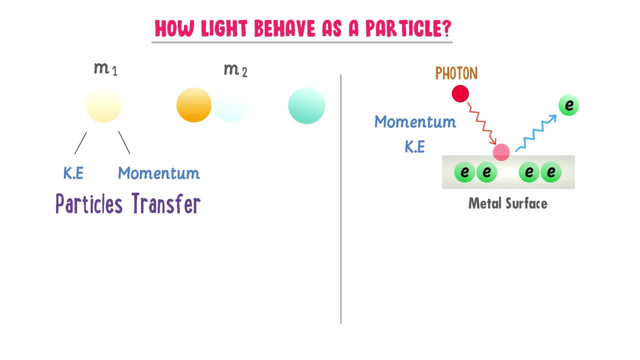 of kinetic energy and momentum. So we say that photons of light also act like a particle, because it can transfer its kinetic energy and momentum. The right-hand side will also transform its energy into the force of the electron. In addition, a particle must also be in the right direction so that the electron may not 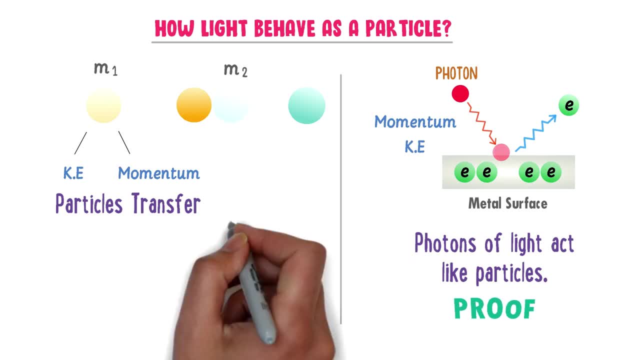 be in the right direction due to the right momentum. Therefore, the right-hand side will also turn into a particle. This is the proof that light also acts as a particle. Now let me ask you one of my favorite questions, which I often ask from my students. 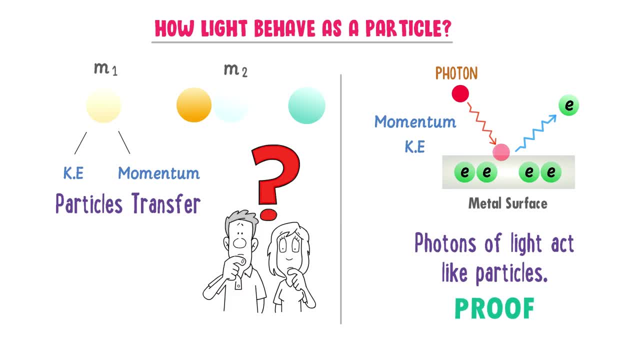 Is light a wave or a particle? The answer is yes. Well, they always say that both Light is a wave and a particle. But I teach them something different. I say that light is not a particle, but is a particle. Whether particle or light, it is a particle. 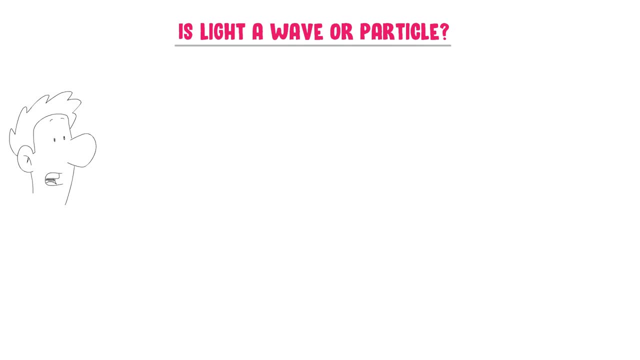 The answer is yes. So if I ask you one more question, which I am often asked, you will say that light is not a particle. even if light is not a particle, Well, they always say that both Light is a wave and a particle. 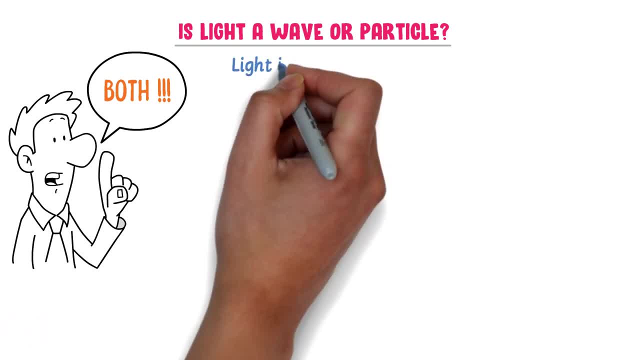 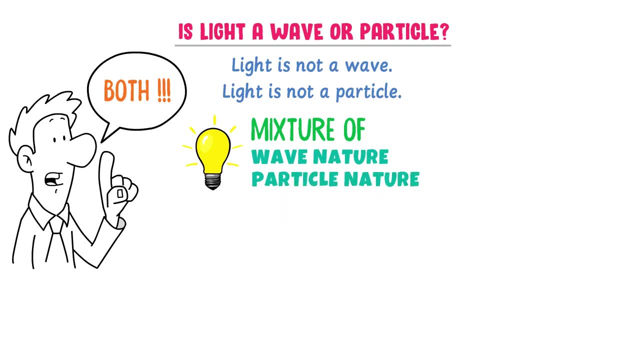 But I teach them something different. I say that light is not a wave, light is not a particle. Light is mixture of wave nature and particle nature. For example, consider this female. If I ask you, is this a man or woman? 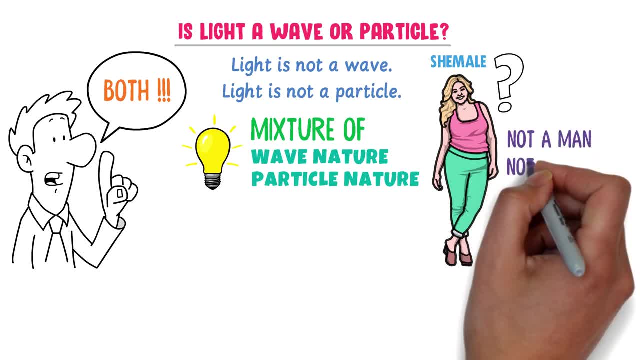 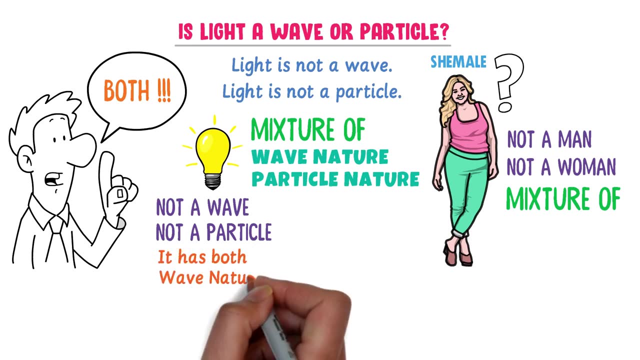 You can say that it is not a man, it is not a woman. She is a mixture of man and woman nature. Similarly, you cannot say that light is a wave, light is a particle. Rather, you can say that it has or carries the wave nature or particle nature. 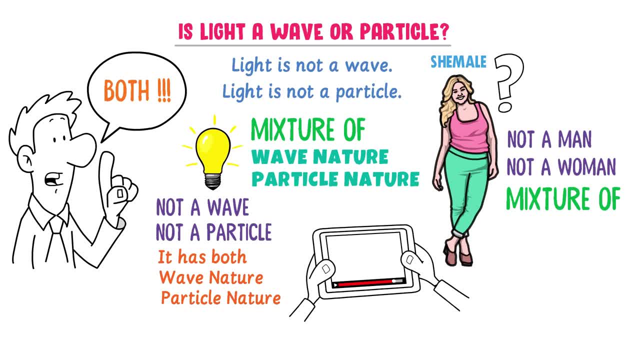 Therefore, you may have seen on the thumbnail that light is neither a wave nor a particle, But it is a mixture of both wave nature and particle nature, just like a female. So always say to yourself: light is a female. Let me repeat it. 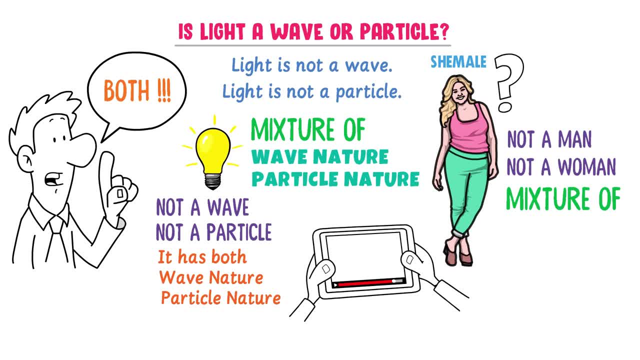 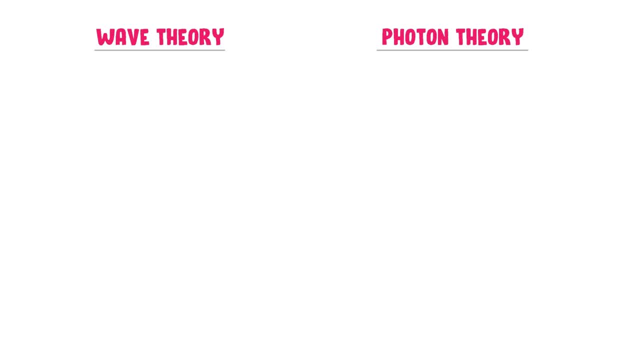 Always say to yourself: light is a female. Finally, let me explain the difference between wave theory of light and photon theory of light. According to wave theory, intensity of light depends upon amplitude. For example, consider these two lights. The amplitude of this light is smaller, so its intensity is lower. 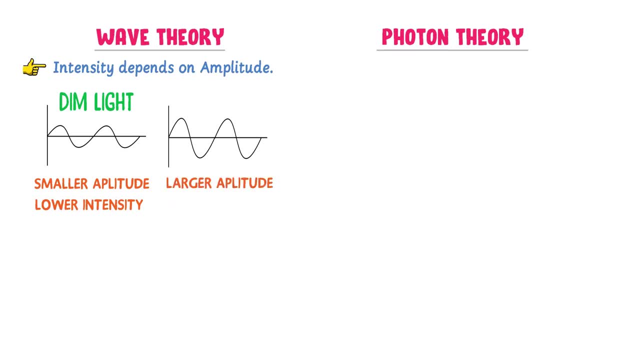 And it is a dim light, While the amplitude of this light is larger, so its intensity is higher and it is a bright light. According to photon theory, intensity of light depends upon the number of photons' arrival. For example, consider these two lights: 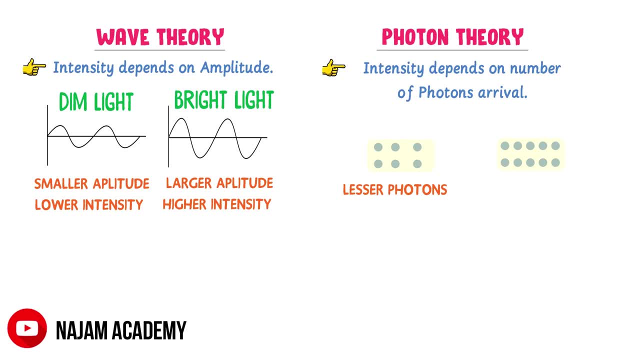 This light has lesser number of photons, so its intensity is smaller and it is a dim light. While this light has larger number of photons, so its intensity is lower and it is a dim light. While this light has lesser number of photons, so its intensity is higher and it is a bright light. 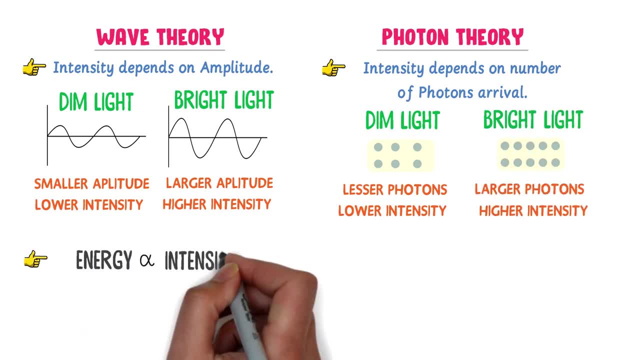 According to wave theory, the energy of light depends upon the intensity. The greater the intensity, the greater would be the energy. According to photon theory, energy of light depends upon frequency. The greater the frequency, the greater would be the energy. Remember that this is totally wrong concept, that